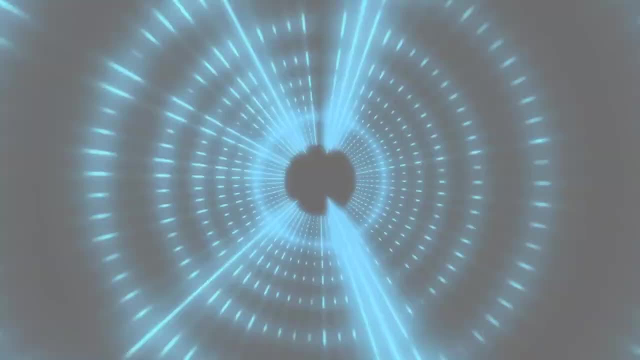 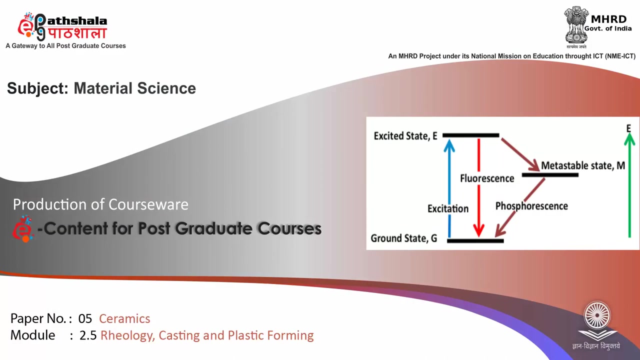 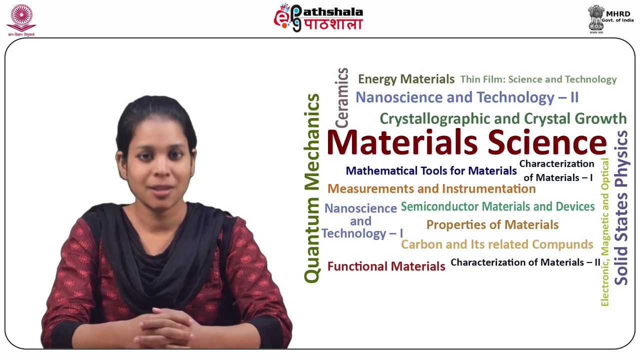 Hello students, welcome to EPG Pardshala. I am Rima Gupta from University of Delhi, and today we are going to discuss about the module rheology, casting and plastic forming, and this is from the paper Processing Ceramics. So, students, let us see what we are going. 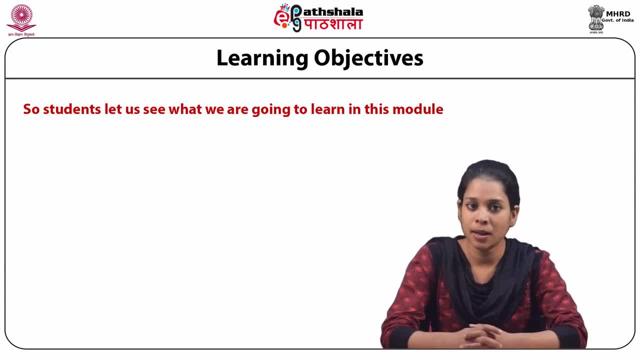 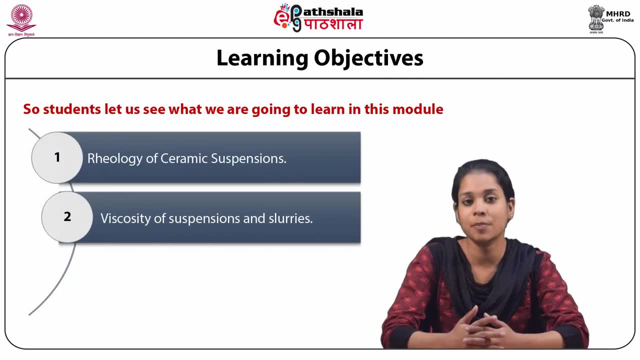 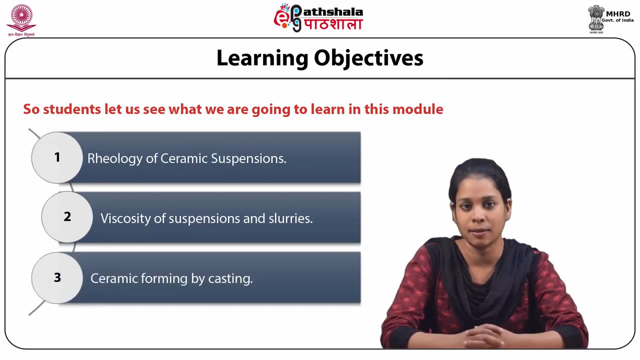 to learn in this module. So first we will be discussing about rheology of ceramic suspensions, then we will be discussing about viscosity of suspensions and slurries and lastly we will discuss about ceramic forming by casting. So before moving in this module, we have discussed. 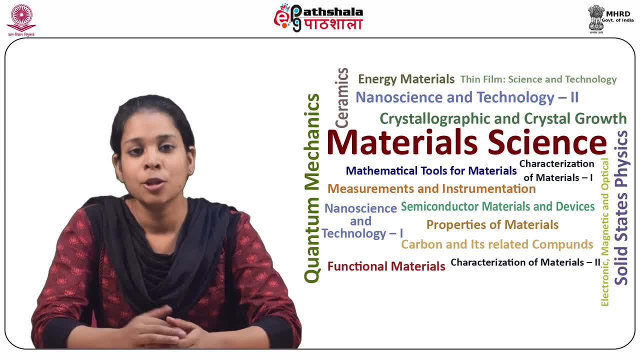 in the previous module regarding dry pressing. So dry pressing is a common method to form a ceramic shapes, So in this case, the dry powder containing small amount of binder is used. The ceramic shapes can also be produced from several other techniques. One of them: 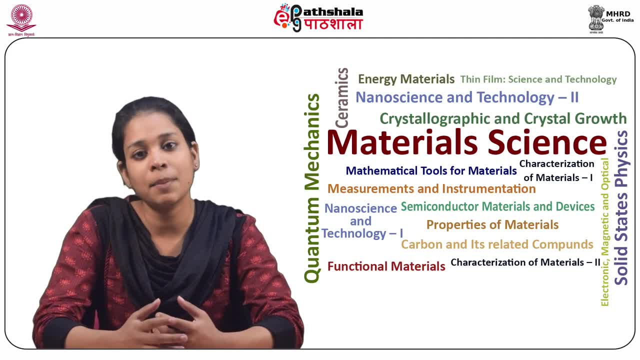 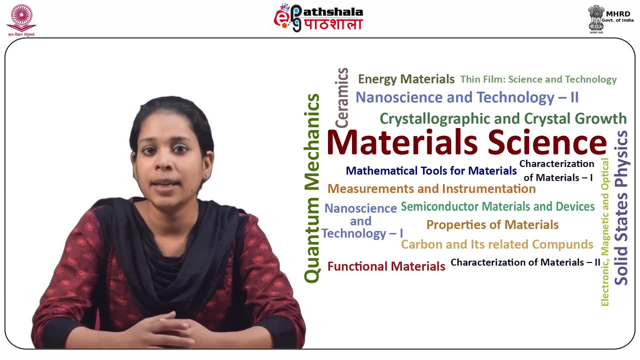 is casting process, in which slurry of ceramic particles is used to cast the required shape in porous mould. The technique that can produce complex shapes as well as massive refractive shapes is this process, and it is also used for advanced ceramic because of the ability to control the agglomerates and uniform mixing of all the additives. So, other than that, 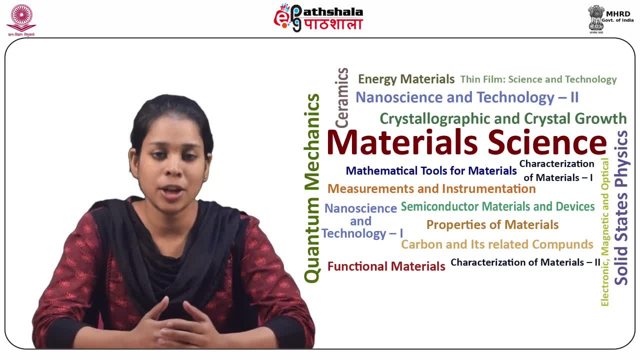 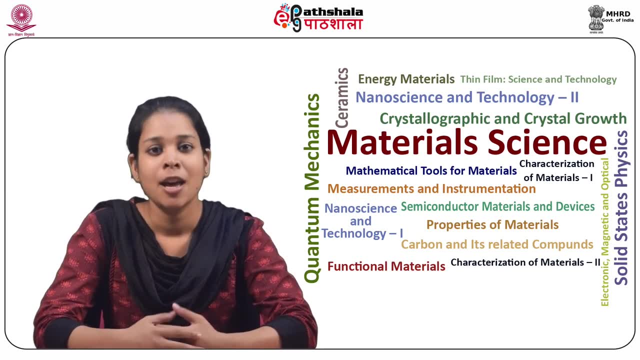 there are various techniques available for shaping it from a paste of ceramic powder, and these techniques include extrusion, injection, moulding. So these forming techniques are discussed in this module and we will be discussing one by one. So first we will talk about rheology. 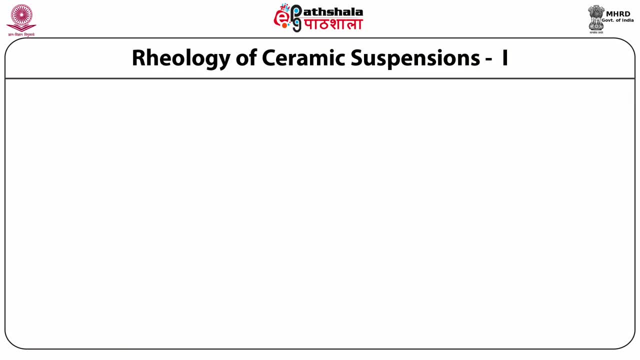 of ceramic suspensions. Rheology concerns itself with the flow and deformation of material. It is of great importance in the casting process. The parameter most commonly measured in the rheological measurements is the viscosity. In ceramic processing with suspensions, slurries and paste, it is essential to know the rheology. Rheology is important in processing as well. 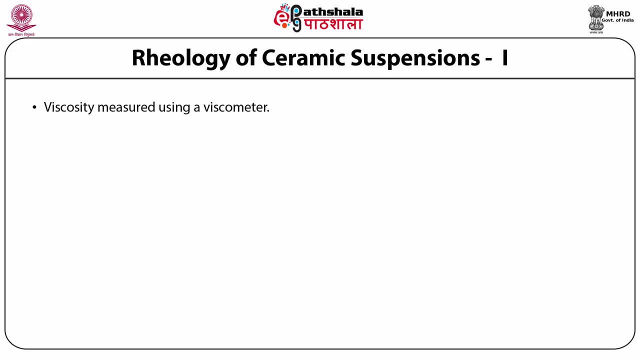 as in operations such as storing, pumping, transporting, mixing, etc. of a ceramic system. A ceramic system, such as suspension or slurry, is a complex system. The rheological behaviour of such a system depends upon the particle size, concentration of the particles in the 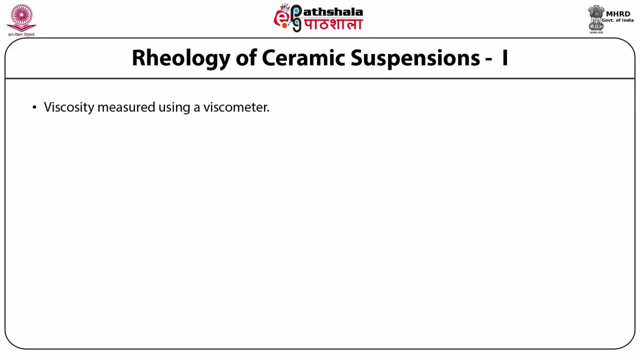 suspension, the interaction present between the particles and other factors. So there are different types of rheological behaviour in ceramic suspension. The viscosity of a suspension is measured by the pressure of the lohngous. The pressure of the lahngous is measured by the resistance at the end of theission. The pressure of the lahngous is: 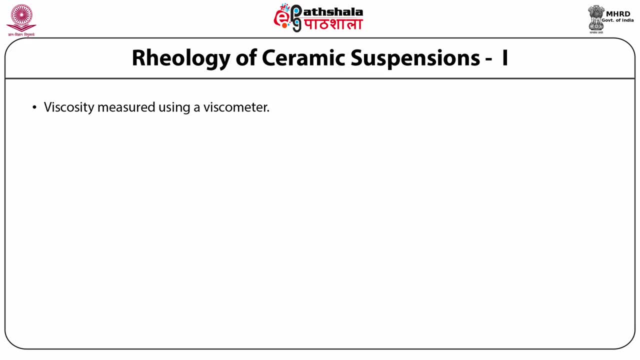 viscometer. the shear rate used for measuring the viscosity can be varied for a given shear rate. a shear stress is applied by the viscometer. the ratio of the shear stress to the strain rate is called the viscosity, or it is given: as tau is equal to eta, gamma dot, where tau is the shear stress and gamma dot is the 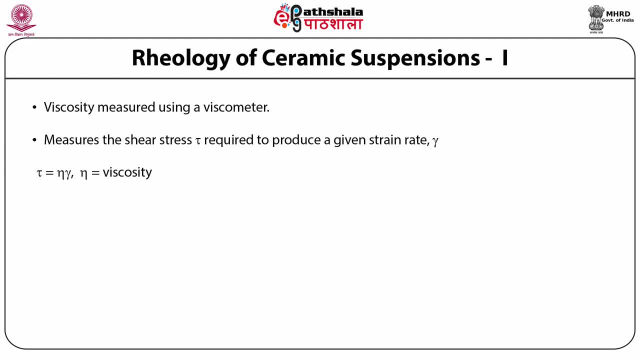 strain rate. it should be noted that the viscosity eta is generally a function of the strain rate, except in one case which is discussed in the next slide. now the rheology of ceramic suspension can be Newtonian type also. so the Newtonian viscous behavior of gamma dot is discussed in this slide. so when the 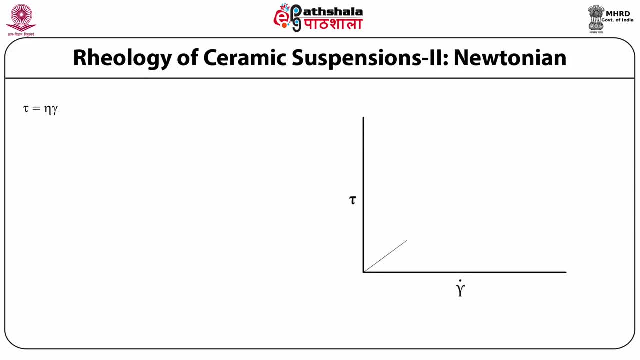 shear stress is directly proportional to the strain rate, then the shear stress is directly proportional to the strain rate at all the strain rates and the constant of proportionality. the viscosity does not change with the strain rate. then the behavior of the fluid is called Newtonian viscous behavior, which is shown in this figure. 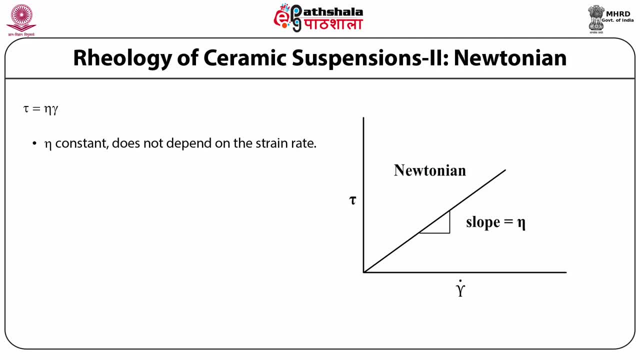 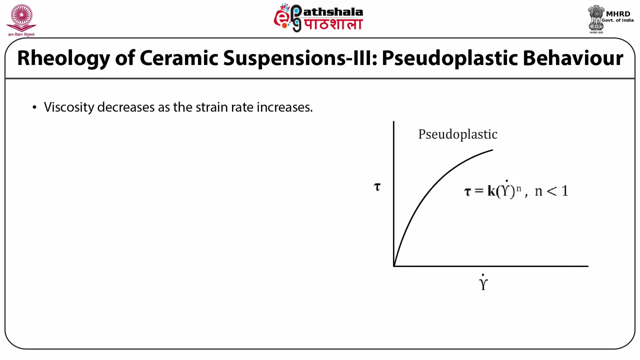 in this case a plot of strain rate versus stress is a straight line. such behavior is found in pure liquids and in dilute suspensions. so the next behavior is pseudo plastic behavior. in this case the viscosity decreases with increasing strain rate. that is the apparent viscosity which is given as eta a that 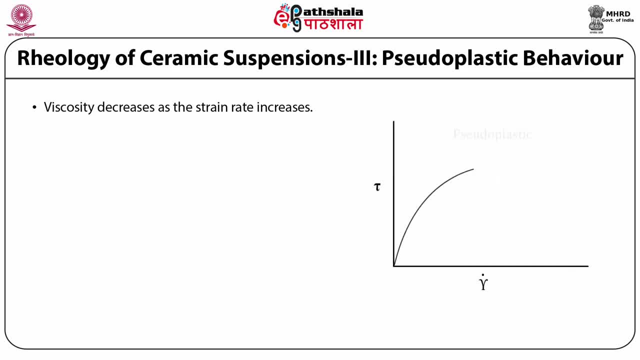 is apparent viscosity is equal to tau divided by gamma dot. so this apparent viscosity decreases as the strain rate increases. a plot of the strain rate is shown in this figure. the strain rate versus stress has a decreasing slope with the increasing strain rate, as shown in this figure. this behavior is found in: 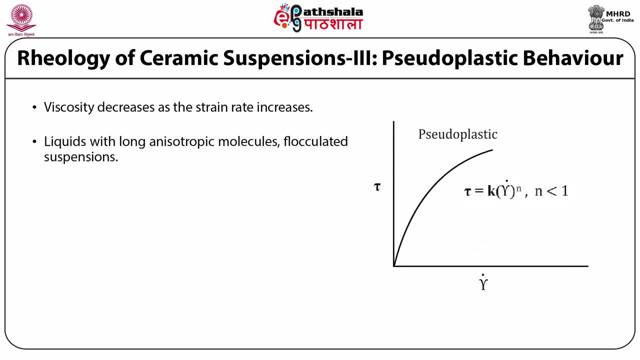 liquids with long and isotropic molecules, suspensions with long particles and in flocculated suspensions. as the shear stress increases, the molecules or the particles get aligned in the flow direction and the strain rate increases. this behavior can also be described by the power law which is stated as tau is. 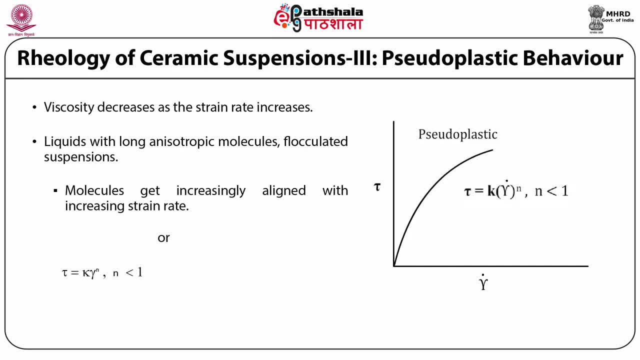 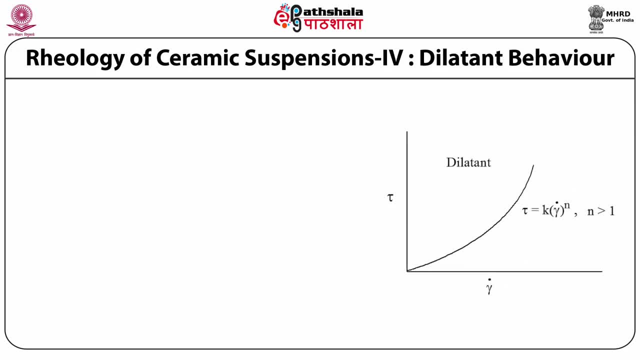 equal to K into gamma dot, to the power n, where n is always less than one. now the next behavior is dilatant behavior. here the apparent viscosity that is eta a increases with increasing strain rate, so that the slope of the strain rate increases. the slope of the strain rate increases the rate of increase in the flow direction. 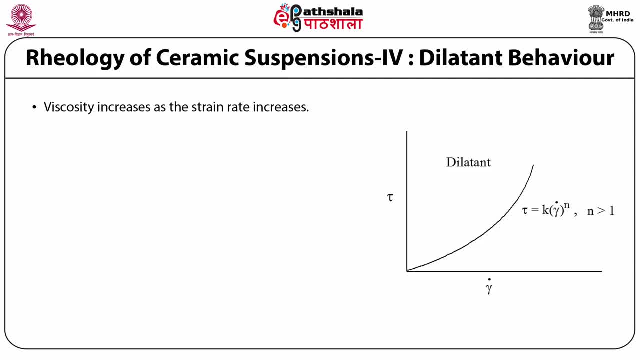 his rate versus shear stress plot increases with increasing strain rate, as can be seen from this figure. This behavior is characteristic of concentrated, defoculated slurries. with increasing strain rate, the particle interference increases, leading to an increase in the viscosity. This behavior can also be described by the power law which we have mentioned earlier. 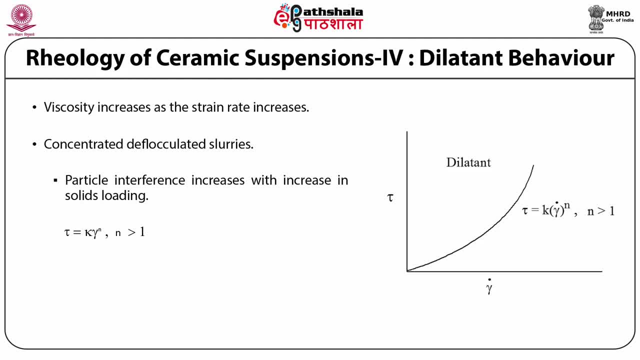 that tau is equal to k into gamma dot, to power n with n greater than 1.. In all the cases which we have mentioned earlier, sometimes the plot does not start at the origin but starts at a finite value of the shear stress, that is, the strain rate remains 0 until the 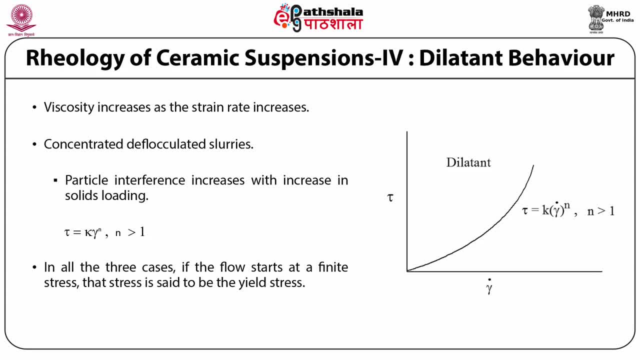 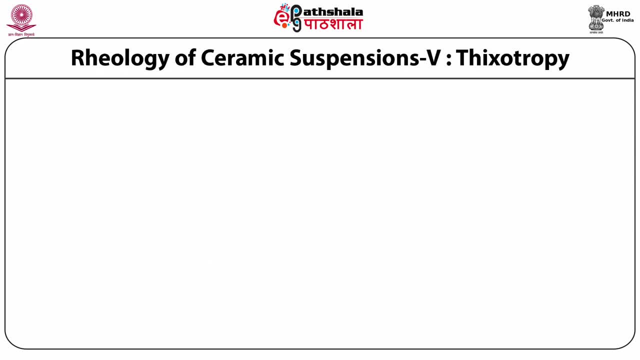 shear stress is increases above a certain value. This value of shear stress is called the yield stress. Now the term comes thixotropy. what is thixotropy? thixotropy is the decrease in viscosity with time while stirring at a constant strain rate. An example is flocculated suspensions, in which 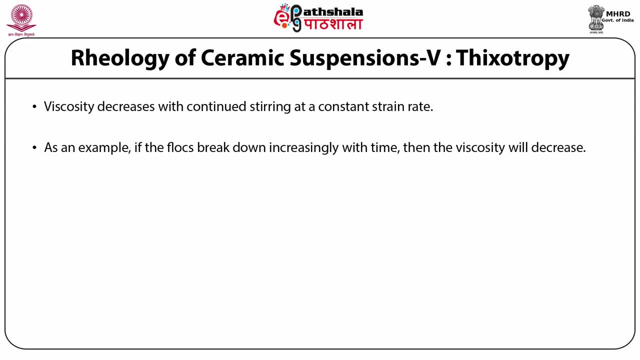 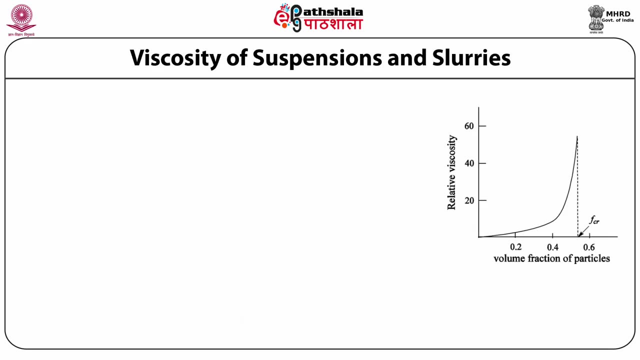 the flocks break with time during stirring, And if the flock break down increasingly with the time will also decrease, as can be seen from this figure, viscosity of suspensions and slurries. so in this slide we will be discussing about viscosity of suspensions of dispersed colloidal particles and viscosity of concentrated 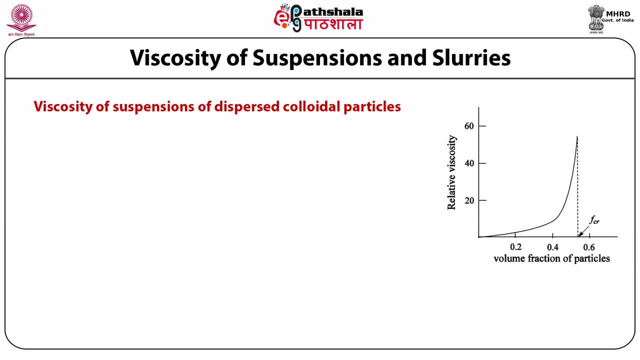 suspensions and slurries. we will first talk about viscosity of suspension of dispersed colloidal particles, in this case a relative viscosity. eta R can be defined as the ratio of the viscosity of the suspension to that of the pure liquid and it is given as eta R, that is, the relative viscosity, is equal to the. 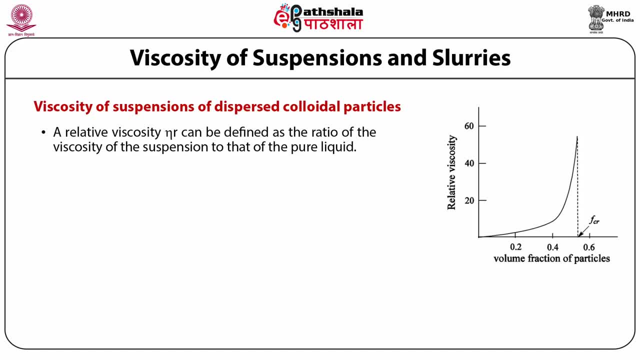 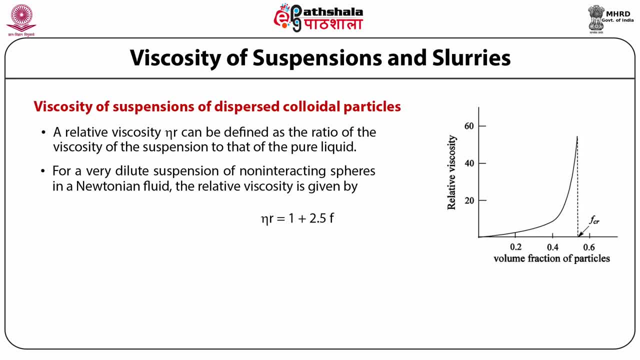 particles. the increase in the viscosity with increasing F is caused by the dissipation of energy as the liquid moves around the particles. this equation is known as Einstein's equation. now, if we talk about non spherical particles, then the constant in this equation, that is, eta R, is equal to 1 plus 2.5 F. the 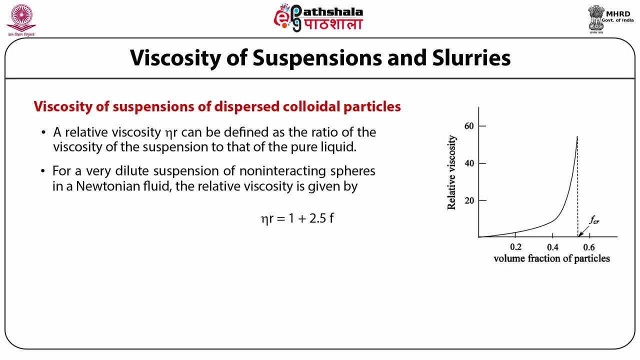 constant is more than 2.5. it will not be 2.5. now we will discuss the second case, that is, viscosity of concentrated suspensions and slurries, the equation which we have described above for relative viscosity. this equation is valid for dilute suspensions when the concentration of particle is. 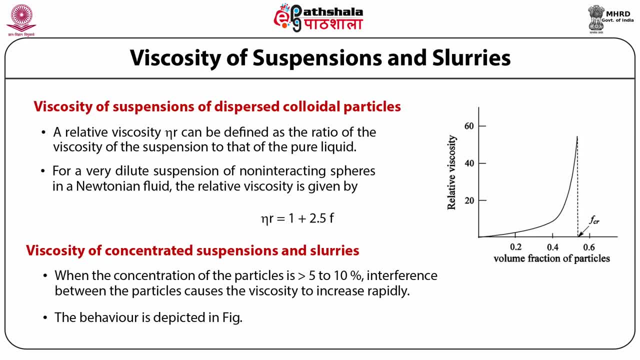 greater than 5 to 10 percent. the interference between the particles causes the viscosity to increase rapidly. the behavior of the concentrated suspensions and slurries can be described as the concentration of the particles which is given. as eta R is equal to 1 minus F divided by F, C, R to. 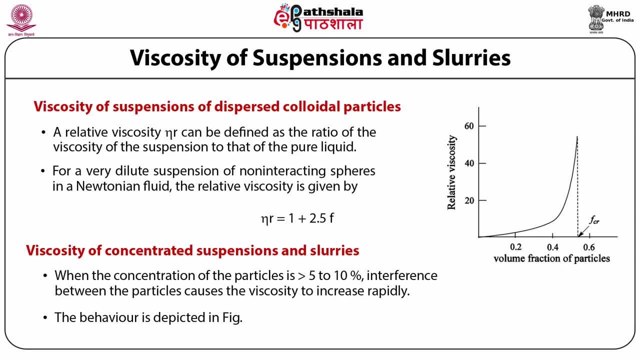 the power K times F C R, where F C R is the critical packing factor at which the flow is blocked and K is a parameter. the behavior can be seen in this figure. as for an aqueous suspension of latex spheres of diameter 0.7 micrometer, it was. 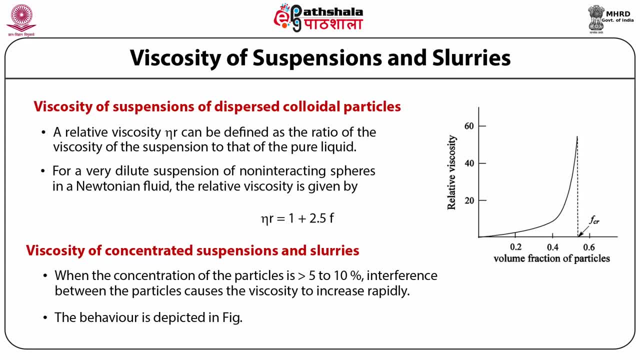 found that K is 2.7, F, C, R is 0.57 to 0.68, depending on the shear rate. the same expression describes the behavior of slurries, which may have particle size distribution ranging from colloidal to a coarse particles. so a simple. 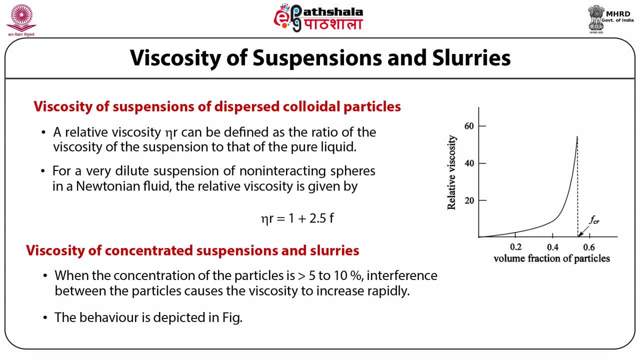 equation can be: etaR is one minus F to power minus K. this equation is used sometimes. in this equation, K is equal to three for a continuous distribution of sizes that pack more efficiently. K is equal to 21 for coarse particles of uniform particle size. now, as I minus F is less. 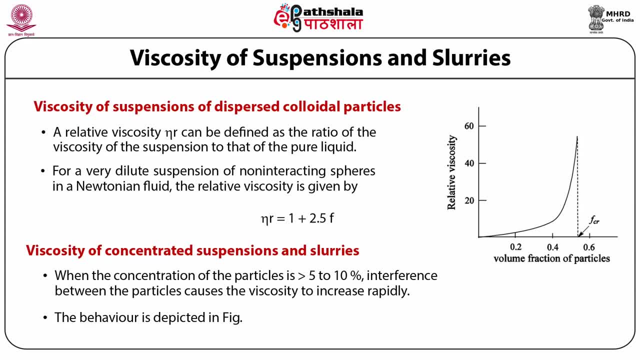 than 1 eta r is higher for the later case. A dilatant behavior can also be observed in concentrated slurries due to mutual particle interference, especially in the case where a high repulsive interaction is present. A dilatant behavior makes the pumping and handling of the 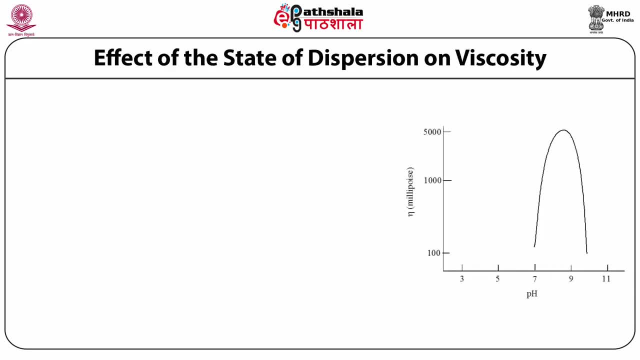 difficult. Now we will discuss about the effect of the state of dispersion on viscosity. The viscosity increases as an initially dispersed systems become more and more foculated. An example is shown in this figure, where the viscosity is plotted as a function of pH. Near the isoelectric point, the aggregation of the particles occur. 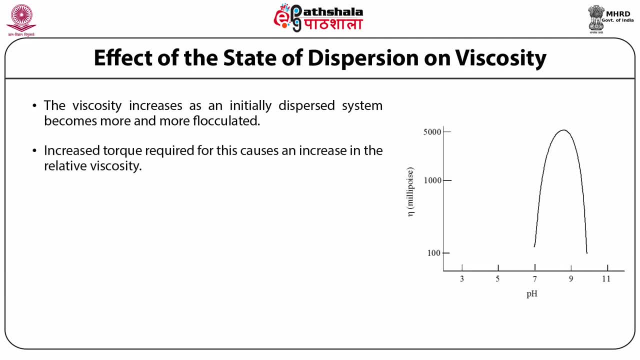 the increased torque required for this causes an increase in the relative viscosity. The flocculated suspensions can be pseudoplastic as an increasing shear rate breaks the flocks to a great extent. It can also be thixotropic if more and more flocks break with continued. 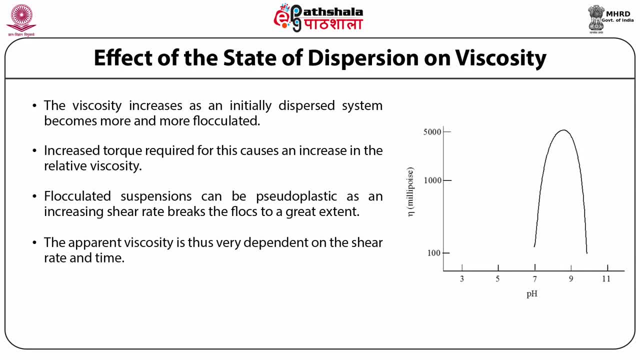 stirring. The epithelial system can also be used as a means of dispersion. The epithelial system can also be used as a means of dispersion. The epithelial system can also be used as a means of dispersion. The apparent viscosity is therefore very much dependent upon the shear rate and time. 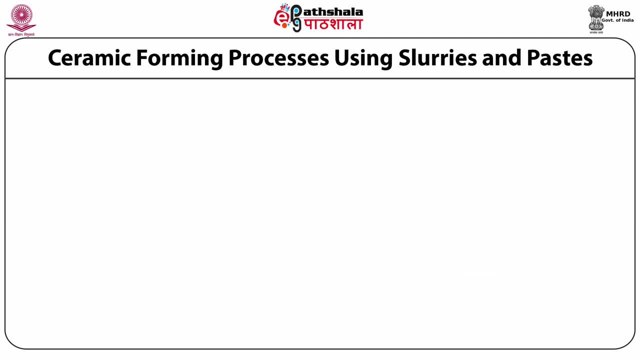 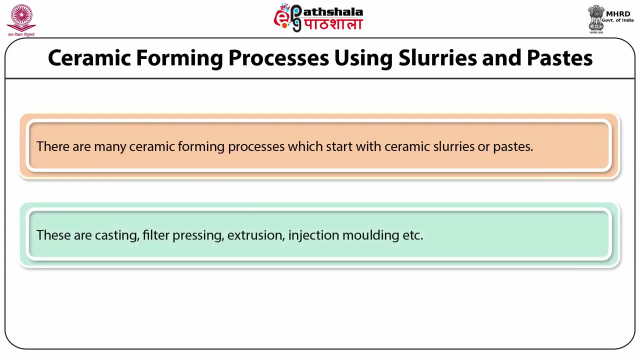 Now we are directing towards the ceramic forming processes using slurries and paste. There are many ceramic forming processes which starts with ceramic slurries or paste. These are casting, filter, pressing, extrusion, injection, molding, etc. We will discuss the all of these one by one. 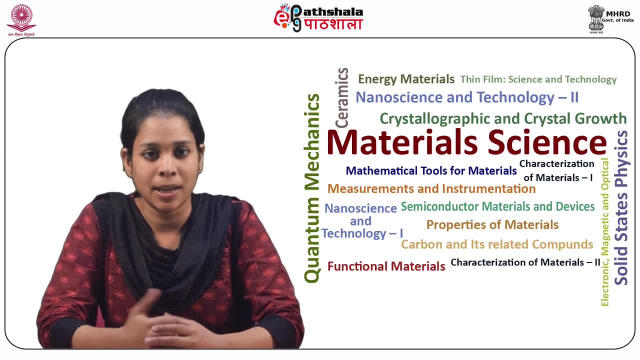 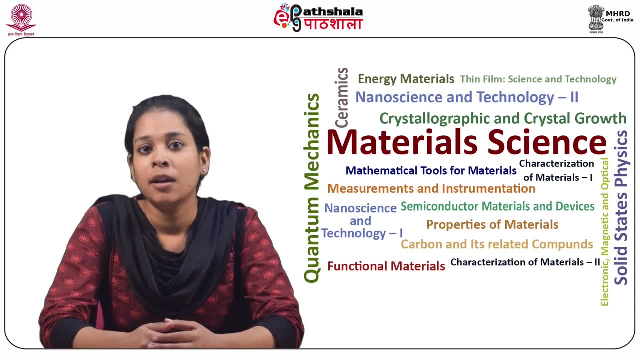 So here comes slip casting. Slip casting is a technique used for manufacturing chemical porcelain, wear refractories having complex shapes or massive in size, sanitary wears, porous thermal insulations, bone china and so on. Slip casting is also used for high performance ceramics with complex shapes. 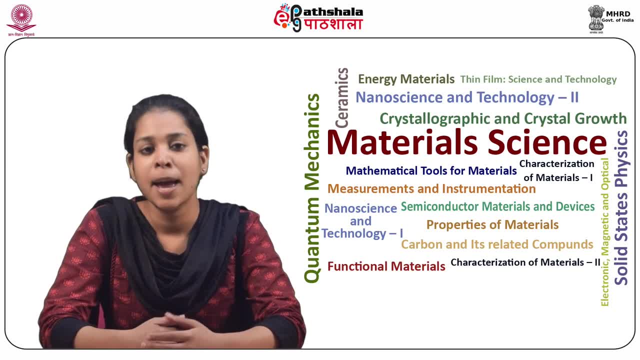 because of the ease of controlling the agglomerates, better mixing of the additives in the slurry and low inversion. So the process essentially consists of preparing slurry of the ceramic to be used and pouring it in a porous mold. The liquid is slowly sucked out through the pores of the mold due to capillary action. 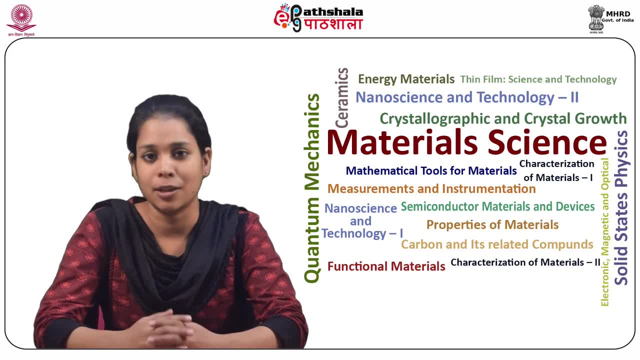 to the external surface where it evaporates. A case of slurry evaporation is a case of slurry evaporation. A case of slurry evaporation is a case of slurry evaporation. The cake is formed adjacent to the internal surface of the mold and the remaining slurry 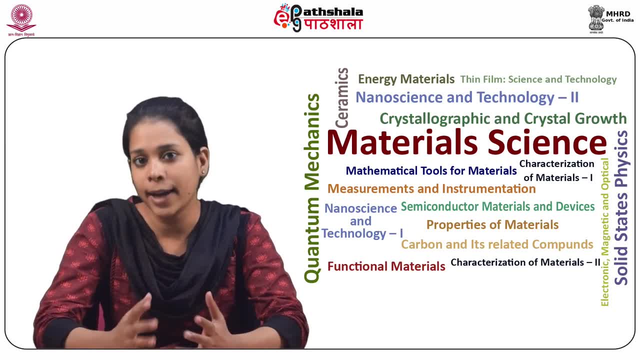 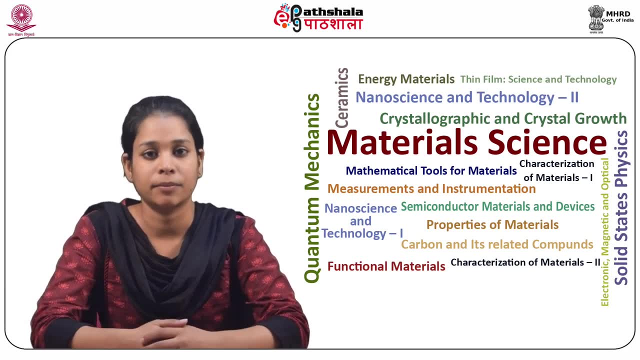 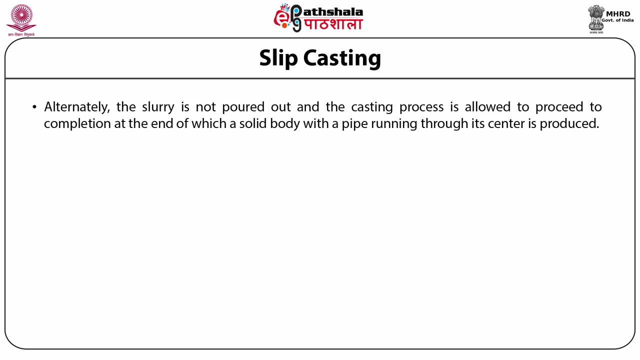 can be poured out of the mold after the required thickness of the cake has formed. So this complete process is called drain casting. So we will start with slip casting. Alternatively, the slurry is not poured out and the casting process is not allowed to proceed. 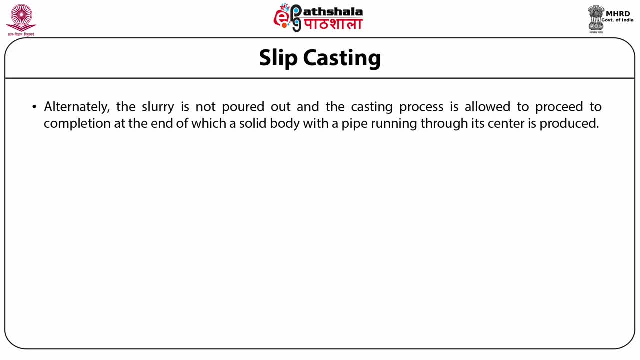 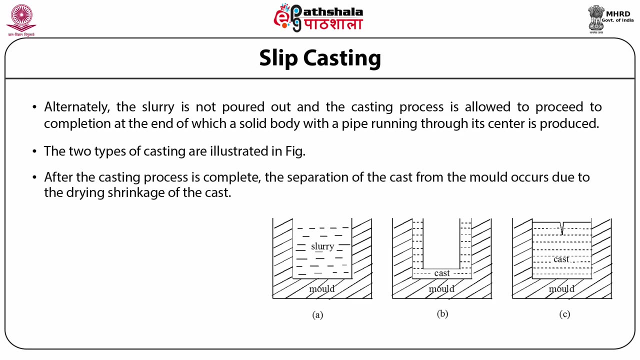 to completion, at the end of which a solid body with a pipe running through its center is produced. This is called solid casting. The two types of casting are illustrated in these figures. After the casting process is complete, the separation of the cast from the mold occurs. 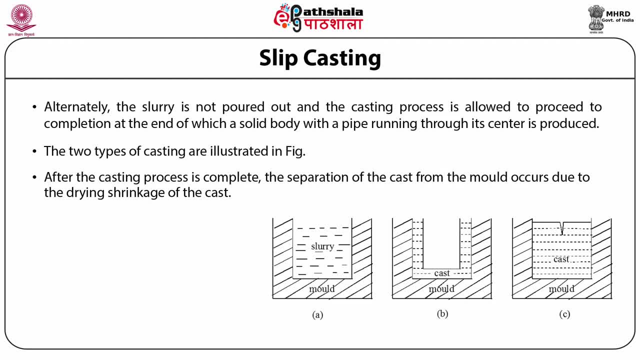 due to the drying, shrinkage of the cast. It may also be affected by blowing air. By blowing air through the mold from the outside, The casting time may range from one hour for a porcelain part within a thin wall to several weeks for a several refractory cast of thickness of 30 cm. 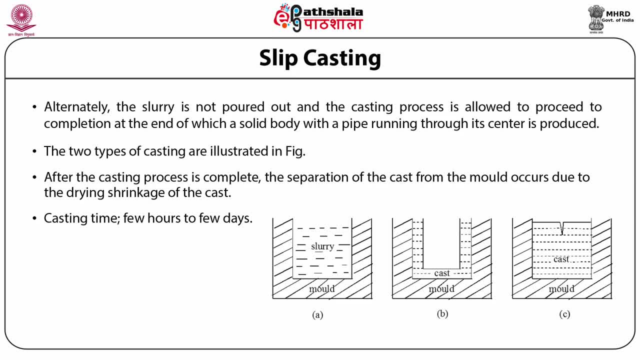 The casting time may be reduced by pressure casting or vacuum casting. The slurry of slip casting can be formulated very carefully to achieve several objectives. These include: the casting rate should be reasonably fast. The cast should have adequate strength for handling subsequent to drying after removal. 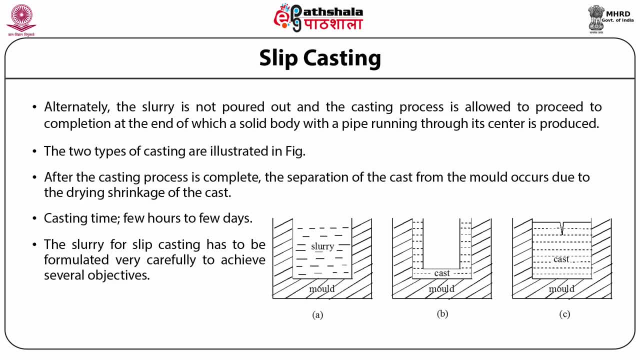 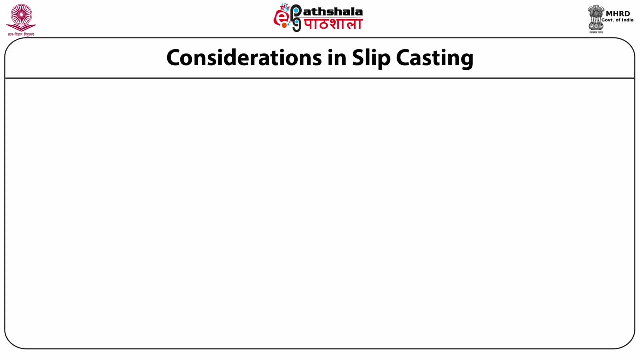 from the mold. And another is the level of porosity in the cast should be as desired. And the last one is the cast should have uniform thickness. Now there are some considerations which we should take into our mind in slip casting. So some factors which are considered while formulating a slurry for slip casting are: 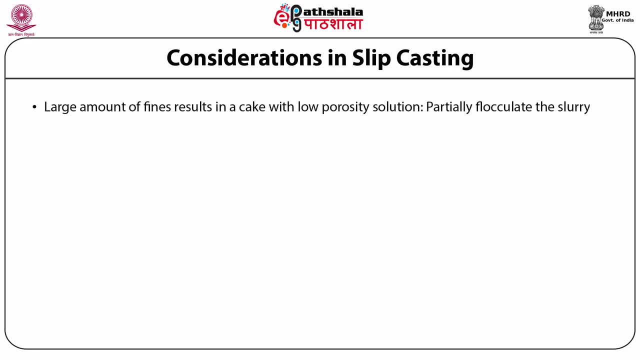 First, a large amount of fine particles in the slurry will produce a cake that has a low porosity, and so the casting rate will be slow and non-uniform. To avoid this, the slurry can be partially flocculated. Second, if the viscosity is too low, such that the particles would tend to settle to the bottom, 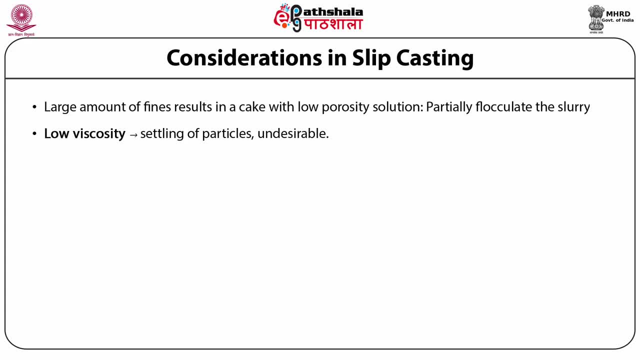 and the available casting time would be small. in slurries with a high viscosity, larger particles can be accommodated. Third, it is desirable to keep the solid loading in the slurry as high as possible so that less liquid has to be removed. The solid loading depends on the thickness of the double layer around each particle. 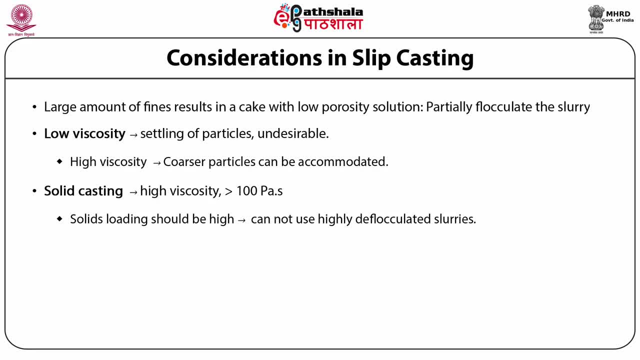 In high deflocculated slurry with fine particles, with each particle having a double layer. the particles cannot be brought closer than a certain distance, and so the solid loading is limited. Fourth, for drain casting, the viscosity should be low, that is, less than 1 pascal second, while it can be greater than. 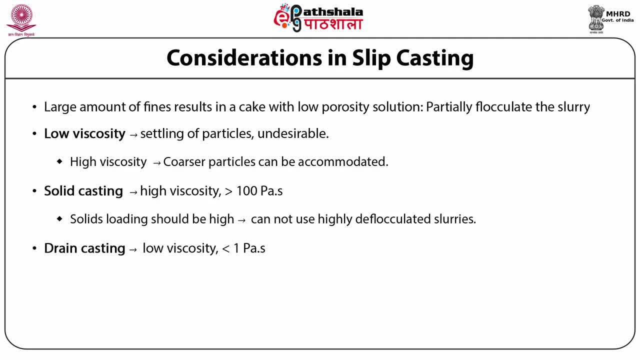 100 pascal, second for solid casting And the last one is the binders are used to provide strength to the cast. Most often, clay is used as a binder. Organic binders of medium molecular weight or inorganic binders are also used. 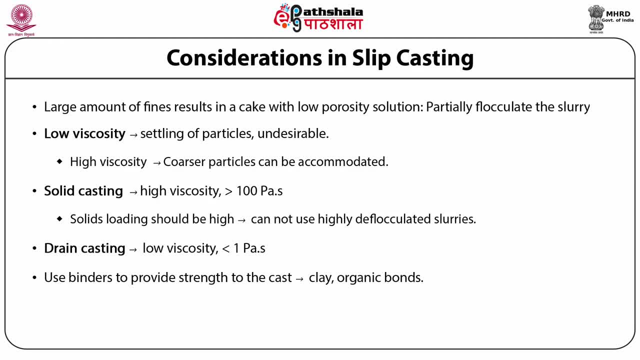 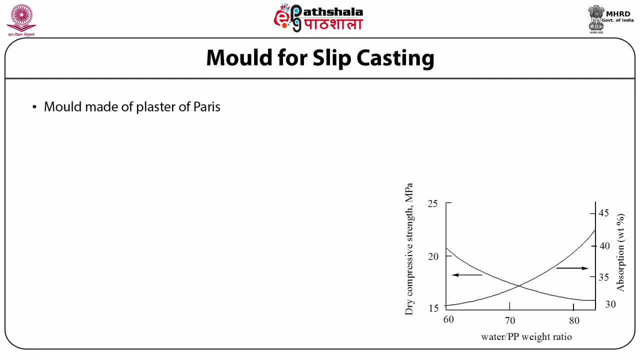 A mixture of binders can also be used instead of clays. The mould is commonly made from plaster of Paris, that is, PP, which is partially hydrated calcium sulphate. On addition of water it gets hydrated to gypsum and the equation is written as follows: and the equation is: 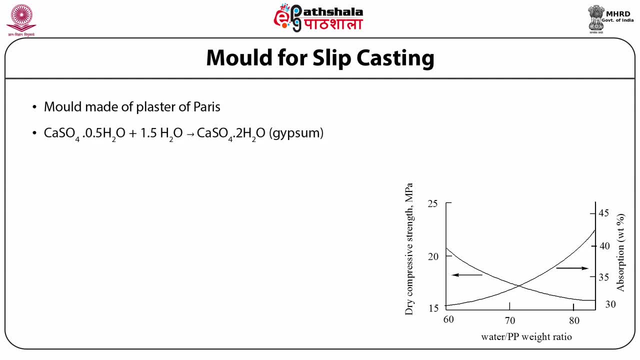 CaSO4.5H2O plus 1.5 times H2O gives CaSO4.2H2O, which is gypsum. The gypsum forms in the form of interpenetrating needles and plates and produces a mould with adequate strength. 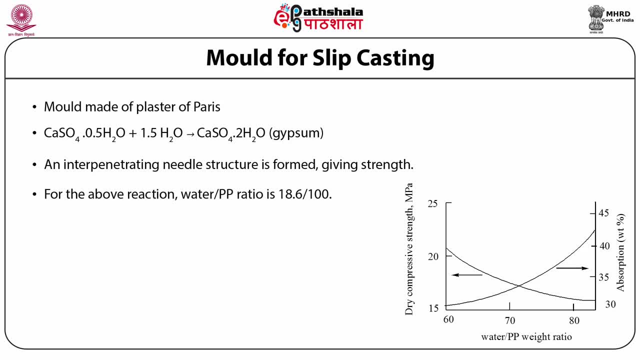 The water to PP ratio, according to the above reaction, is 18.6 by 100. So a range of 60 by 100 to 80 by 100 is used to produce the mould to give adequate porosity, The variation of the strength of the mould and its water absorption capacity with water. 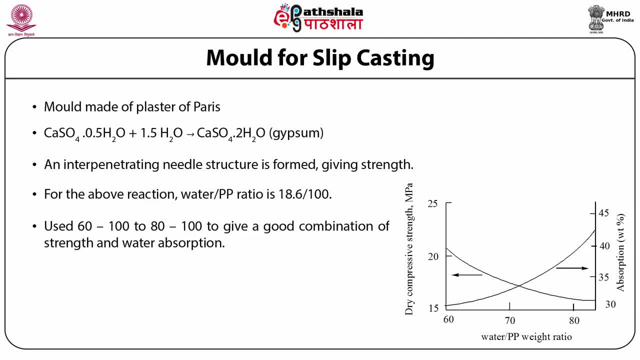 to plaster ratio is also shown in this figure. The liquid being removed from the slurry has to pass through the cake, which forms a slurry. The slurry has to pass through the cake which forms a slurry. The slurry has to pass through the cake which forms a slurry. 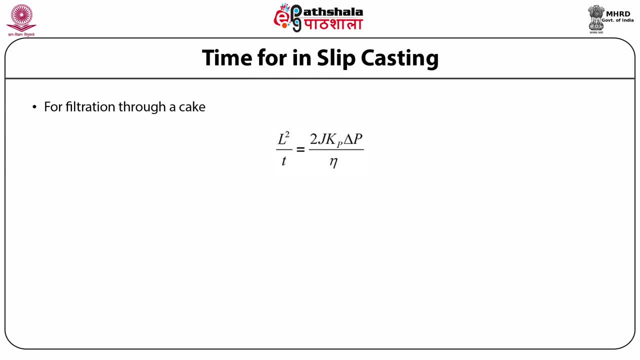 The slurry forms on the wall of the mould, The cake acts as a filter. The uniaxial flow rate through a filter is proportional to the difference in pressure of delta P across the filter, with thickness L and cross-sectional area A. So the equations become: Q is equal to KD A-delta P divided by L, which can also be reduced to. 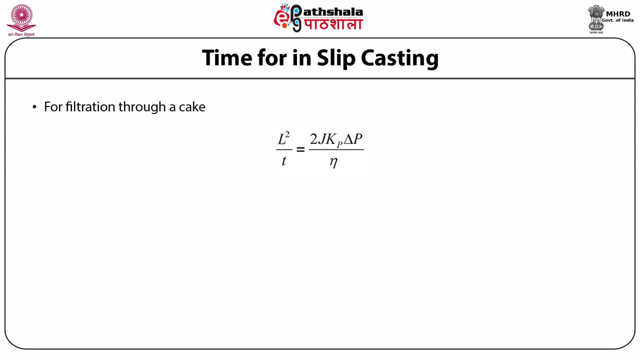 which can also be written as KpAΔp, divided by ηL, where Kd is the DRC permeability coefficient and η is the viscosity of filtrate. Moreover, Kp is the specific permeability For the filtration. through a cake, one gets the formula as: 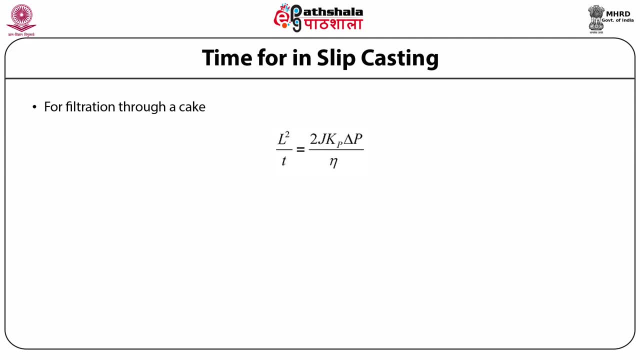 L2 by T is equal to 2JKpΔp divided by η, where L is the thickness of the cake produced in time, T, J is the volume of the cake per unit. volume of the filtrate. This equation shows that the thickness of the cake increases as the square root of the time of casting. 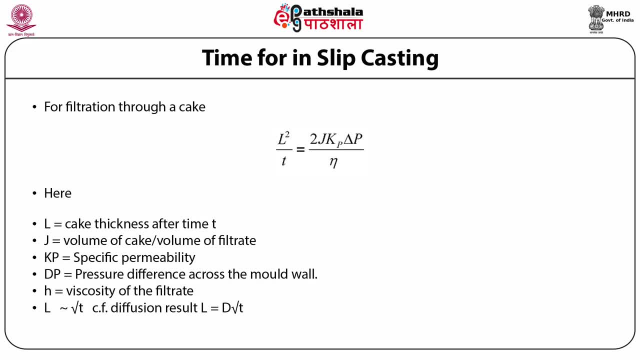 and it is similar to the difference Diffusion equation, which is: L is equal to D times root T, where L is the thickness through which the diffusion of the specie takes place in time, T and D is the diffusion coefficient. Now the next process is tape casting. 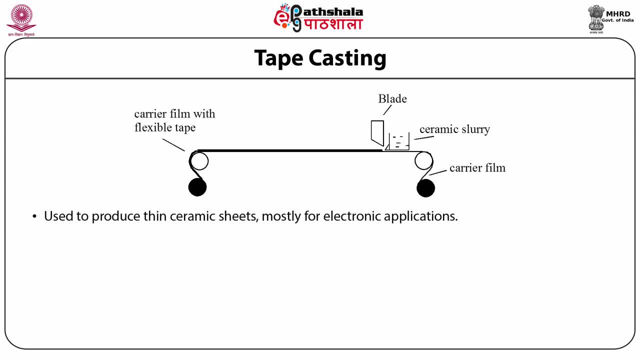 The tape casting process is used to produce thin. thin means less than 1 mm, So to produce thin ceramic material, we need to use a thin metal sheet, A slurry made in organic solvents like tri-chloroethylene or ethanol and containing substantial amounts of organic binders. 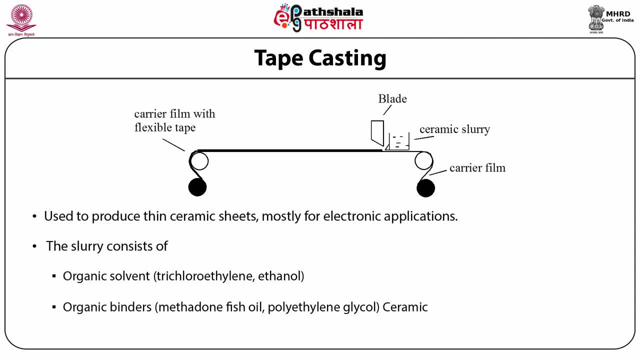 example, methadone, fish oil, polyethylene glycol, etc. is poured over a flat surface and a sharp blade with a small clearance position over the surface seen in this figure. This produces a thin layer of constant thickness. The thickness of the layer. 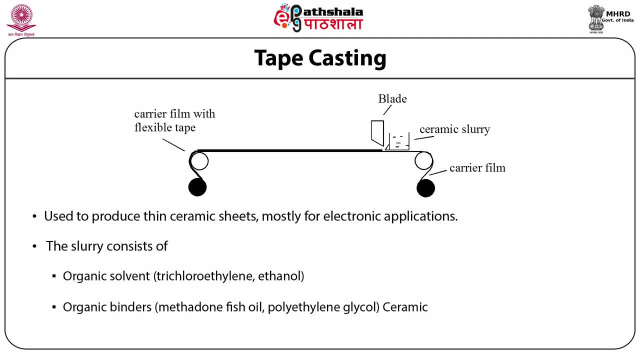 can be controlled by controlling the cap between the blade and the casting surface. Upon drying, the sheet becomes leather-like and can be slit, punched, etc. before sintering. This process is used to produce multi-layer capacitors, substrates of electronic packaging, etc. 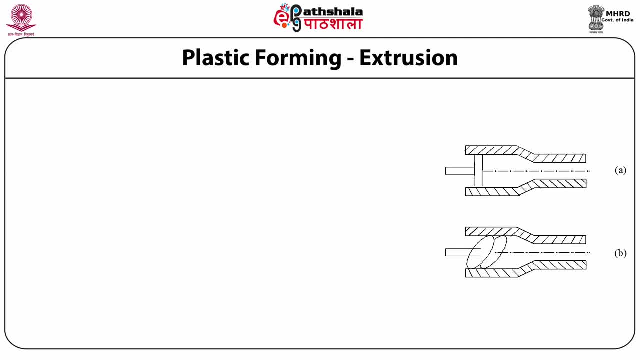 Now we will discuss the plastic forming. So the mixture of clay and water produces a plastic mass, as we all know, which can be shaped by deforming into the desired shape. Processes like extrusion, plastic pressing, jiggering, have been traditionally used to shape clay bodies. A plastic mass can also be produced by mixing any ceramic powder. 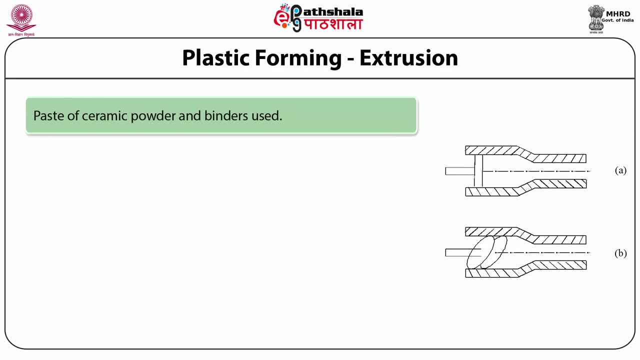 with clay or organic binders, and the same process can be used to produce the part of that ceramic. So we will first discuss the extrusion. In extrusion, the plastic mass is forced through a rigid die having a desired cross-section. The process is used to shape the clay bodies. So we will first discuss the extrusion. In extrusion, the plastic mass is forced through a rigid die having a desired cross-section. The process is used to shape the clay bodies. So we will first discuss the extrusion. The plastic mass is forced through a rigid die having a desired cross-section. 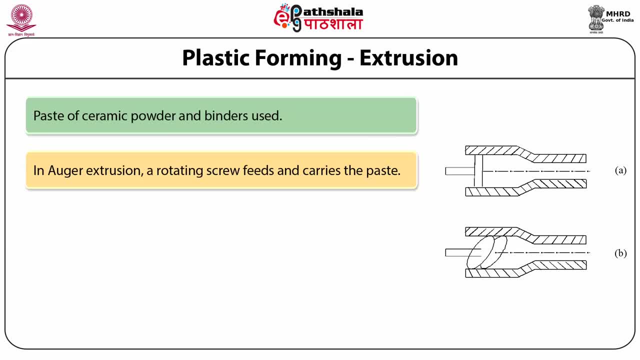 The products made by extrusion include a variety of refractory and porcelain products of complex shapes, such as hollow surface tubes, honeycomb catalyst supports, transparent alumina tubes for lamps, flat substrates, etc. So the two types of equipment which are used for 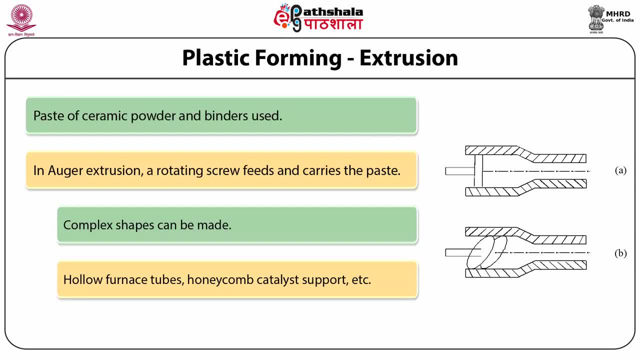 So the two types of equipment which are used for extrusion are groundwood and redwood. So the two types of equipment which are used for extrusion are groundwood and redwood. extrusion are discussed below. In one, the plastic mass is pushed by a piston inside a barrel and 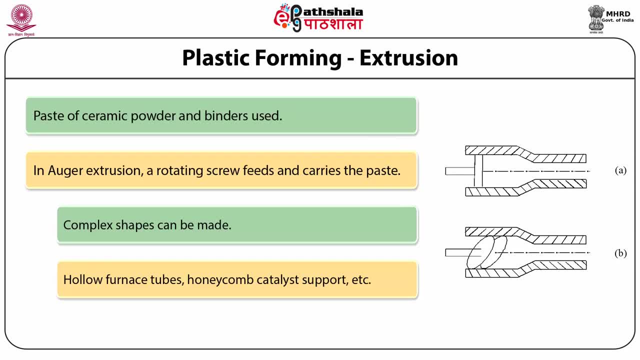 through a die, which is shown in figure A. This is a batch process in which feed material is fed intermittently, and in the second type of equipment the feed material is fed and carried in the barrel by a rotating screw called an auger. This is also shown in figure B, The arrangement of auger extruder. 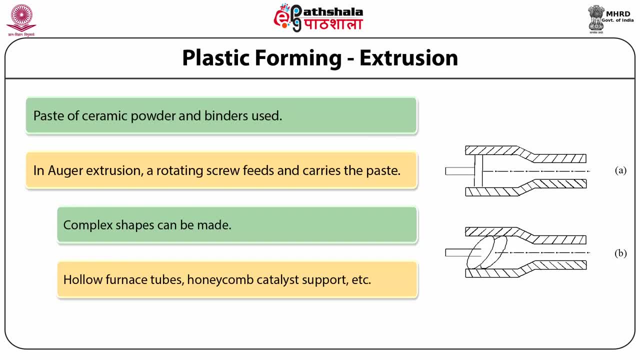 is shown in this figure also, The pressures used in a piston extruder is about 4 MPa for porcelain bodies and about 15 MPa for organically plasticized bodies. This can be compared to the pressure of about 200 MPa. 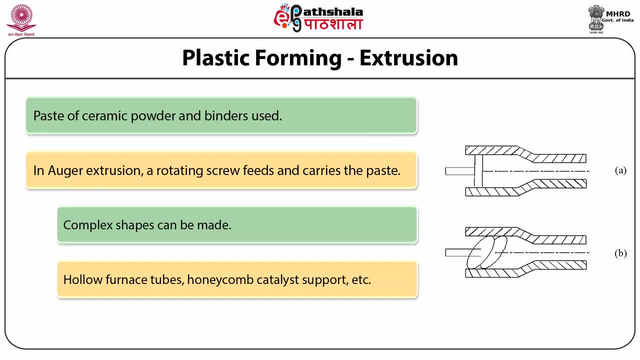 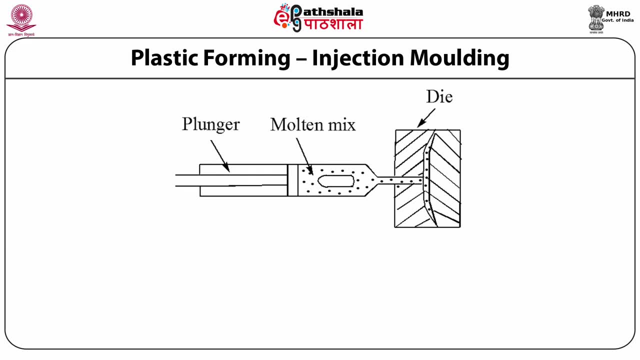 Now the next is injection molding, which is a type of plastic forming, As mentioned earlier. in injection molding, a molten thermoplastic heavily doped with ceramic powder is injected into a die, as shown in this figure. It is a rapid process and can produce complex shapes with a lot of pressure. This is a 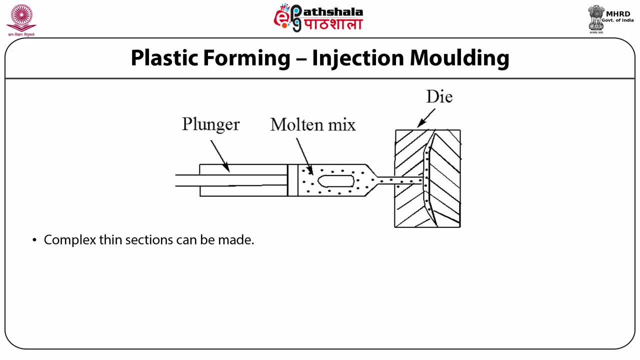 illustration of a process of injection molding. So in injection molding the thermoplastics are preferred over thermosets because of the factors such as storage, stability and reusability of the scrap. Two types of thermoplastics are generally used. One is called. 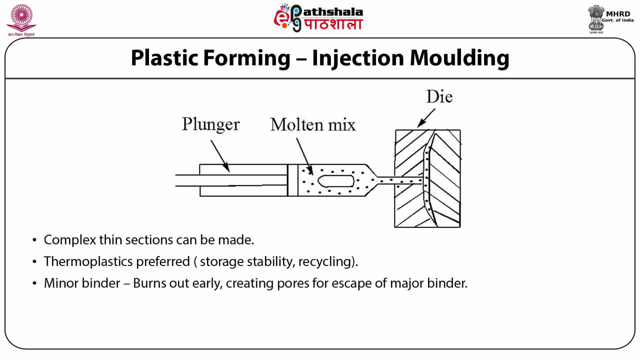 minor binder which, during the post-forming removal of the polymer, burns out earlier, and provides pore channels for the inside of the trap. As mentioned earlier. these are for steamers escape of the major binder which burns out later. In addition to the binders, a plasticizer or we 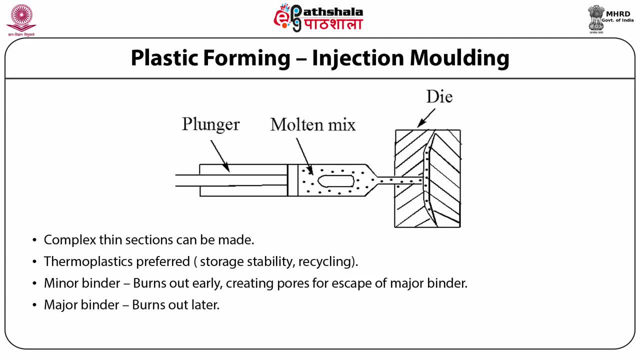 can say lubricant and a surfactant for particle wetting are also used. Some of the examples of major binder are high molecular weight polythene and the example for minor binder is parafilm wax, etc. The temperature used during injection molding is about 125 to 150 degree Celsius. 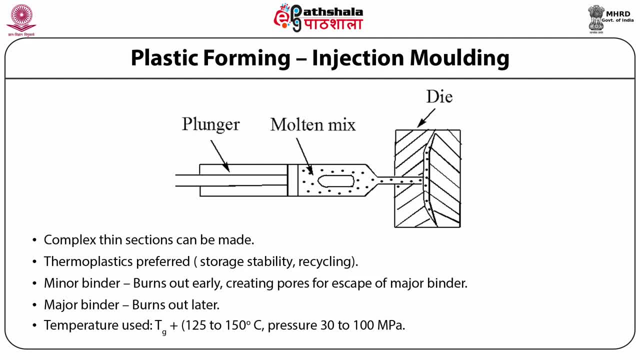 higher than the temperature Tg of the major binder. The pressure used is 30 to 100 megapascal and during injection molding, maintaining suitable temperature at each location is very critical process. The parts with complex shapes, dimensionally accurate and with smooth surfaces can be produced by injection molding. The 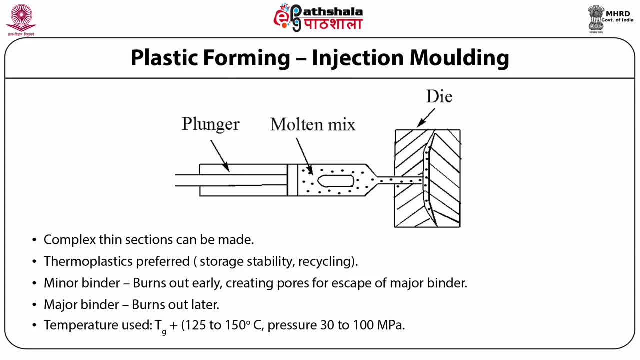 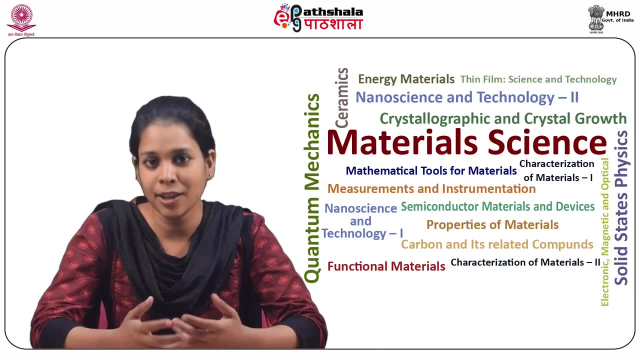 tolerance is thickness, which is around 0.5 to 5 mm, and the holes smaller than 1 mm can be produced with a tolerance of less than 0.1 mm. So, students, let's summarize what we have learned in this module. So first we have read about casting and plasticization. 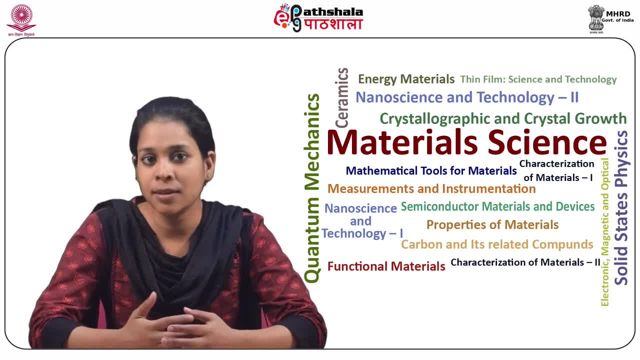 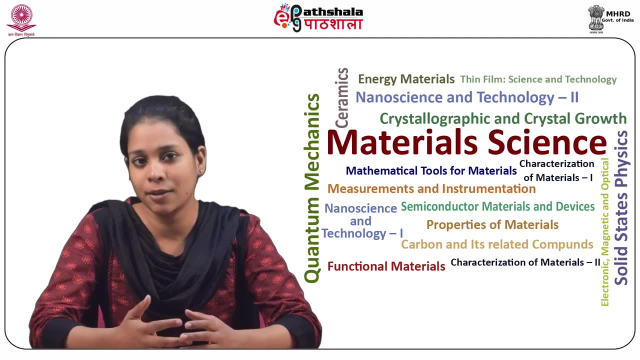 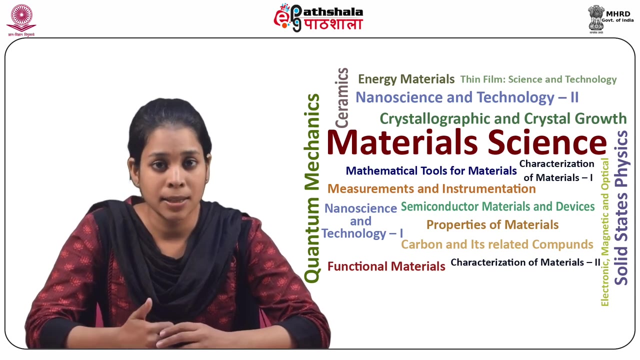 Then we have discussed the first process, that is, casting, where we have learned that rheology is very much important. Next, we have read about pseudoplastic behavior, in which the viscosity decreases with the strain rate which is desirable for casting, And in slip casting, a slurry is poured into a porous mold made of plaster of Paris. This is the process. 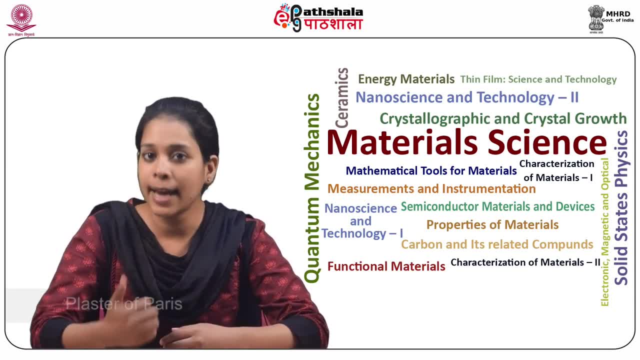 that we have learned in this module. So we have discussed the first process, that is, casting, where we have learned that rheology is very much important. Next, we have read about pseudoplastic behavior, in which the viscosity decreases with the strain rate which is desirable for.